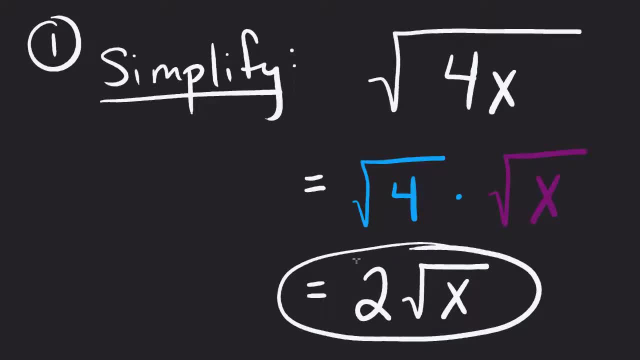 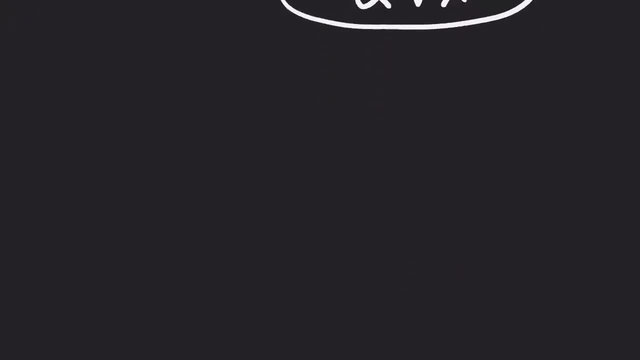 We've now simplified this problem, So what it allows us to do is separate, simplify and then come up with a final solution. All right, so let's try one that's a little bit trickier, a little bit harder to see. 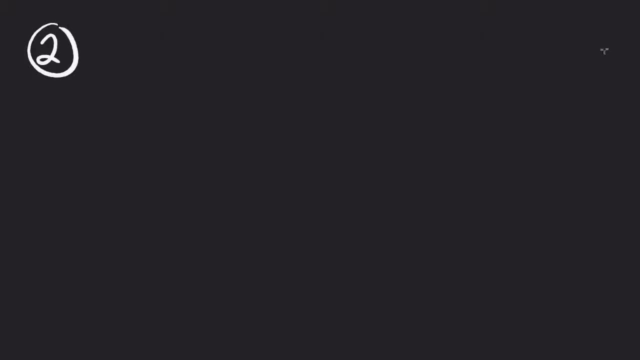 And these are the ones that we'll probably use. We'll probably use more of as we get further along. So let's look at something like this: Simplify the square root of 72.. All right, these numbers come up a lot when we get these big square roots. 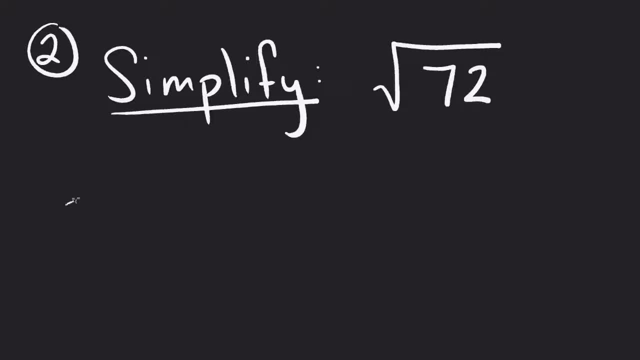 We're not exactly sure what to do with them. Well, what we could do, though, is we can do it several different ways, but this is one way we can use this property. It's to separate this into. It's to separate this into 36 times square root of 2.. 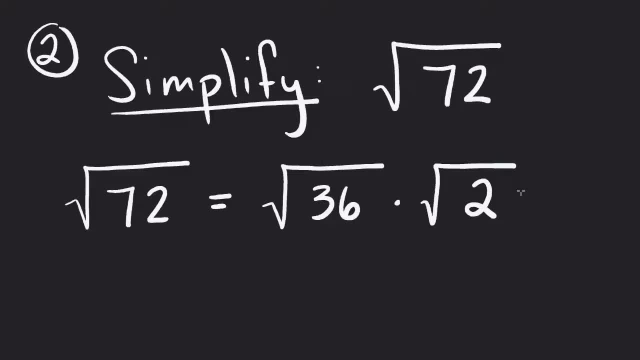 So we've got the square root of 36 times the square root of 2, which is 36 times 2 is 72. So 36 turns out to be a perfect square. So this one right here will actually simplify into 6.. 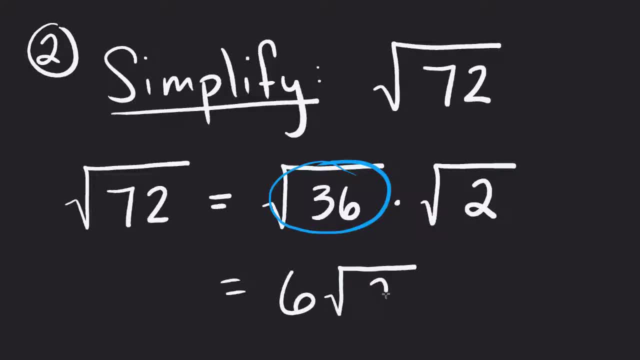 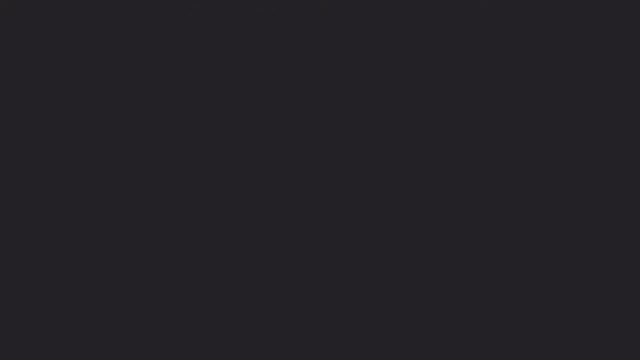 And the square root of 2 cannot simplify, so we end up with 6 square root 2.. So we could use this for other examples. We can exactly look at this one, actually in a different way. So let's say that we looked at this same problem. 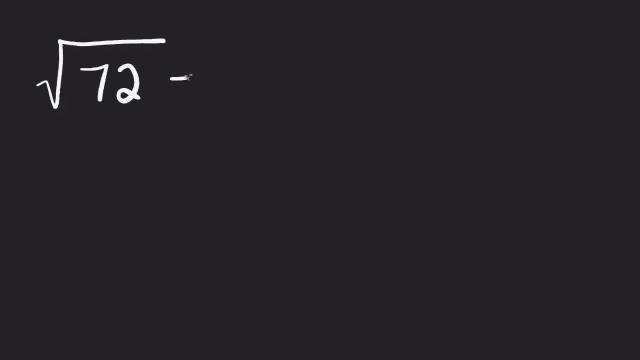 I want to make sure you see, kind of, how this works. Let's see a different way of looking at this problem. So let's say that I saw this as Well. this is 2. times 4 times the square root of 9.. 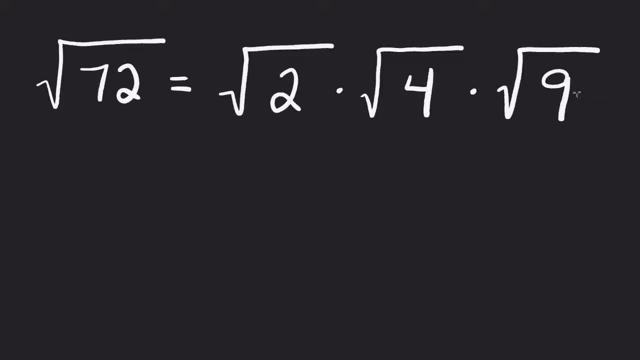 Okay, so let's say that I broke this down into smaller numbers and I happen to see that, Well, again, this one will simplify and this one will simplify. So let's see what those give us. So the square root of 2 can't simplify. 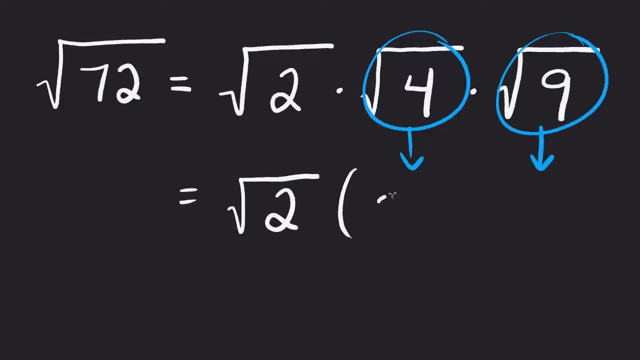 because we don't have a pair, The square root of 4 turns out to be 2. And the square root of 9 turns out to be 3.. So when we clean this up and we kind of simplify this out together,